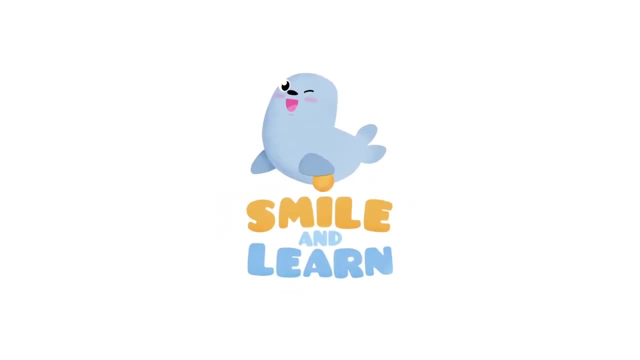 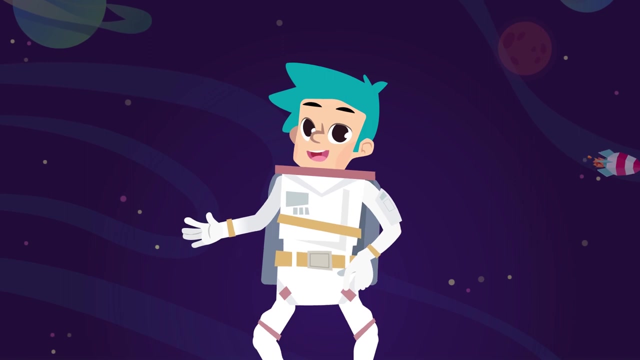 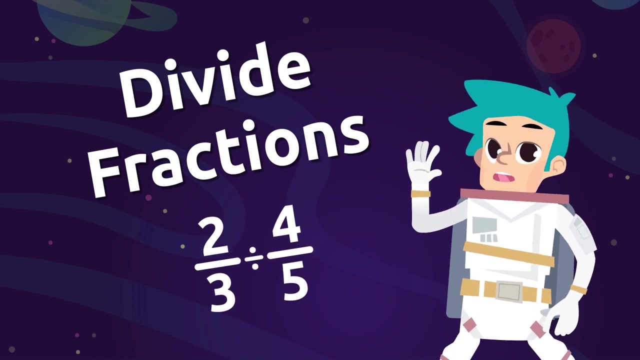 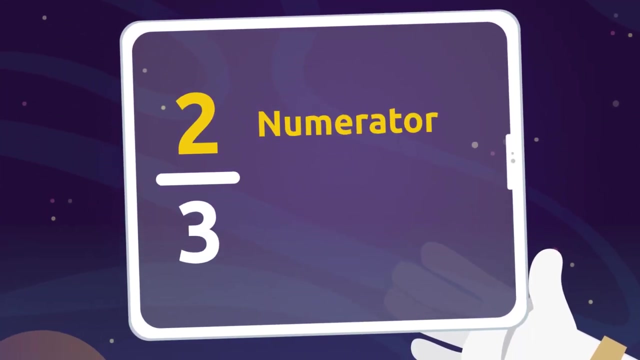 Hello again, friends. We continue practicing operations with fractions. Today we're going to learn how to divide fractions. First, let's recap quickly the parts of a fraction. The top number is the numerator and the bottom number is the denominator. Now we're ready. 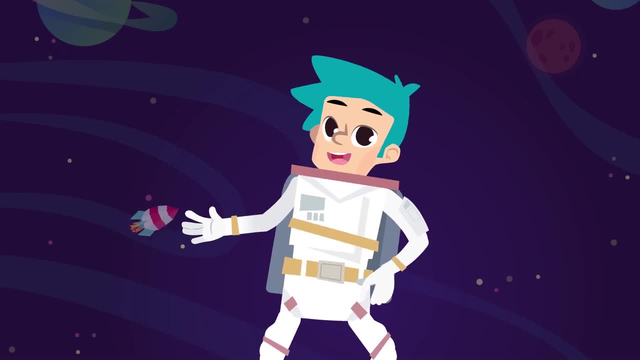 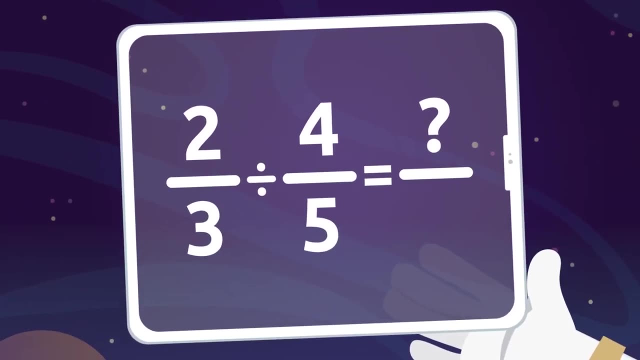 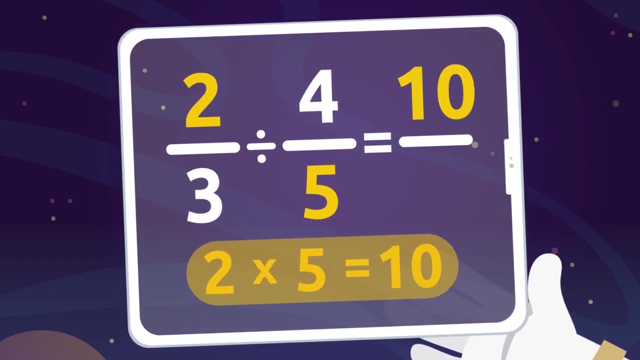 to start. Dividing fractions is fun. Do you want to know how it's done? When we divide fractions? to find the numerator, we should multiply the numerator of the first fraction by the denominator of the second fraction. To find the denominator, we multiply the denominator. 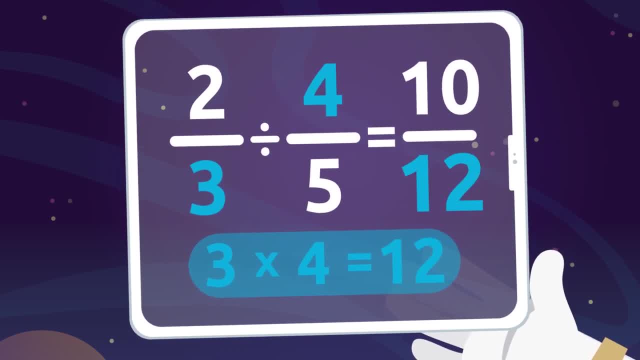 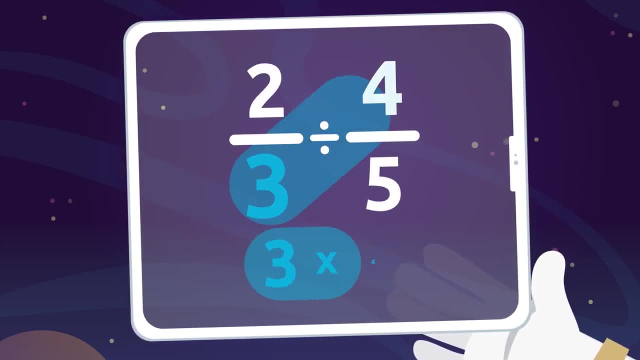 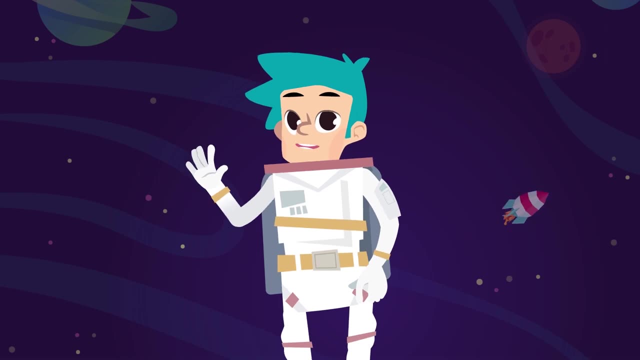 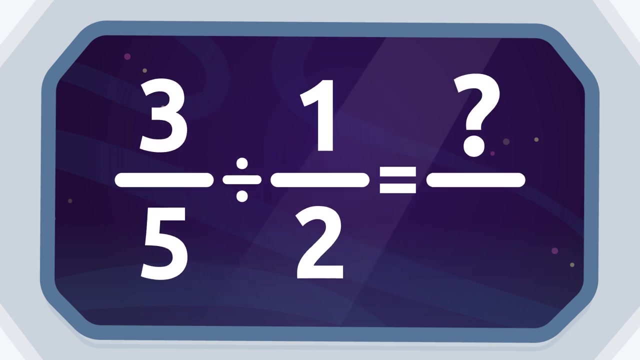 of the first fraction by the numerator of the second fraction. This means that to divide fractions, we cross-multiply them. Did you understand how it's done? Let's look at the next example. We need to divide three-fifths by one-half To find the numerator of the. 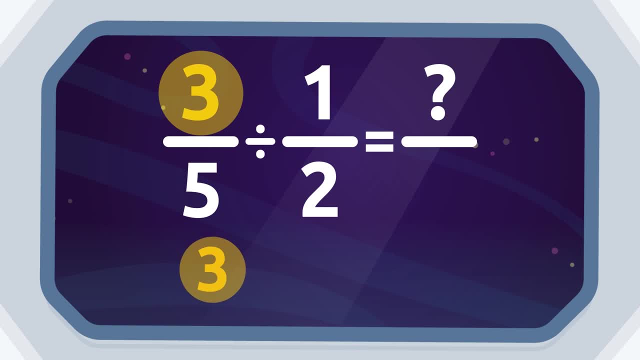 product. we multiply the numerator of the first fraction by the denominator of the second fraction, meaning three by two, which equals six. The numerator of the product is six. so we multiply the denominator of the first fraction by the numerator of the second fraction. 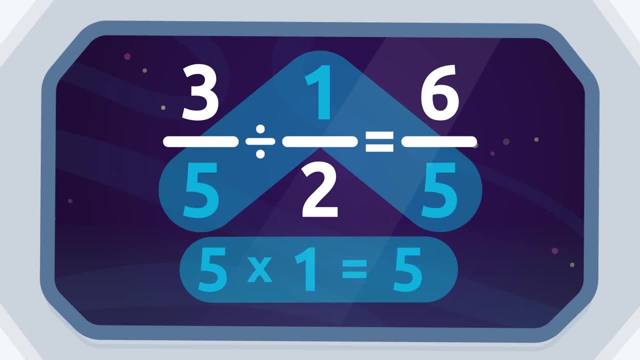 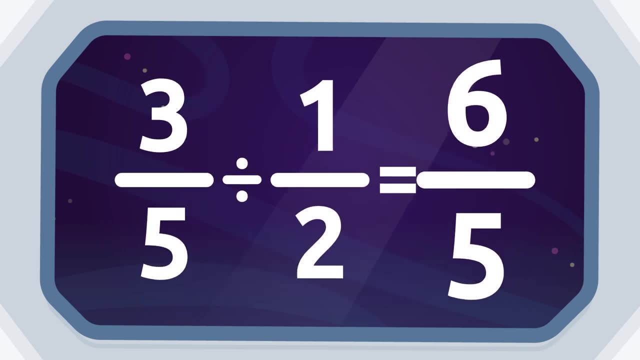 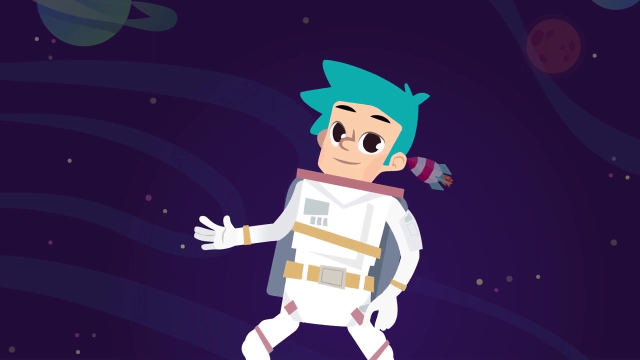 meaning five by one, which equals five. The denominator of the product is five, so three-fifths divided by one-half equals six-fifths- Excellent. Let's look at the next example. Would you like to try doing this one yourself? 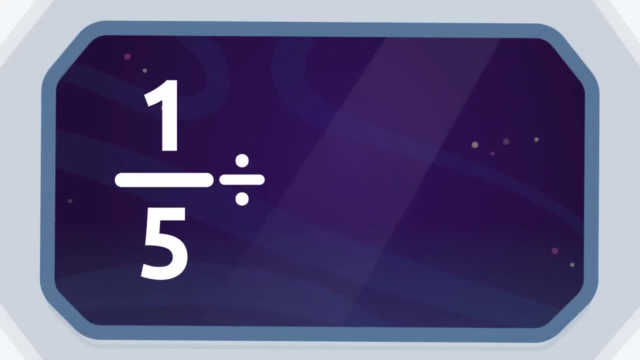 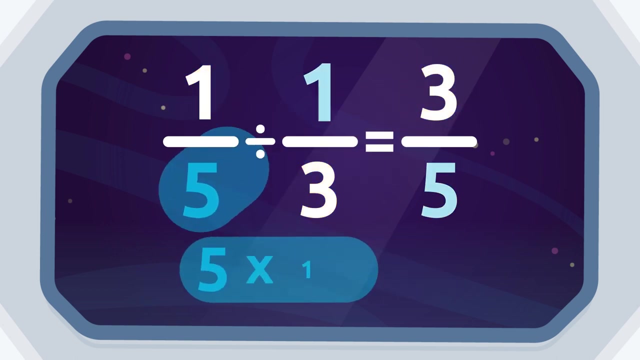 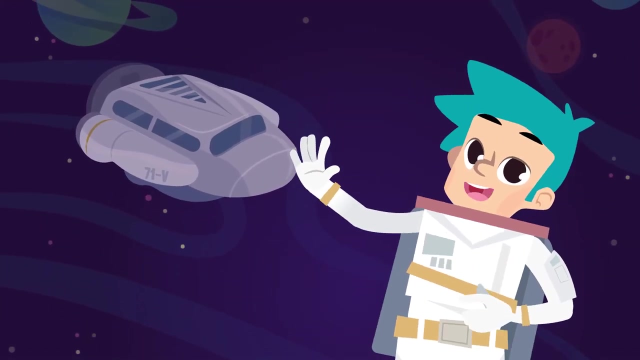 One-fifth divided by one-third equals: Let's find out if you got it right. One-fifth divided by one-third equals three-fifths. Great job, Congratulations. Now you know how to divide fractions. You're a real expert, See you. on the next video.